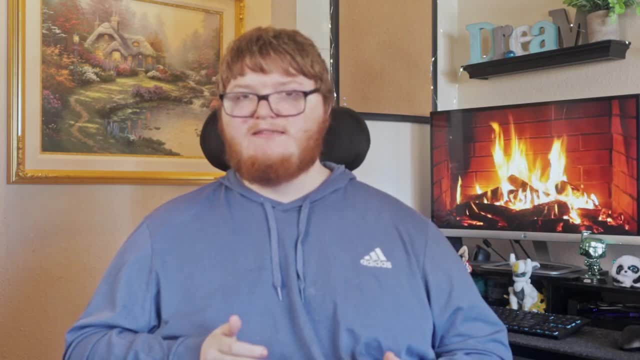 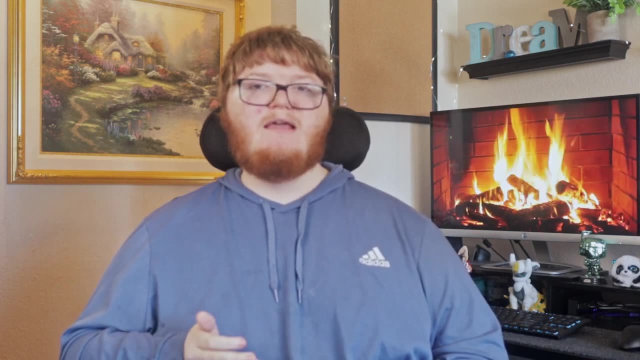 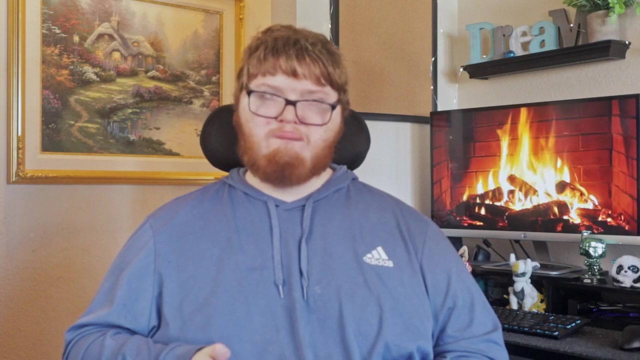 two fundamentals, as each of them have a hard time existing well without the others, Without world building, there's nowhere for your story to take place. World building doesn't even have to be anything new. You could do world building in earth as we know it right now, if you really. 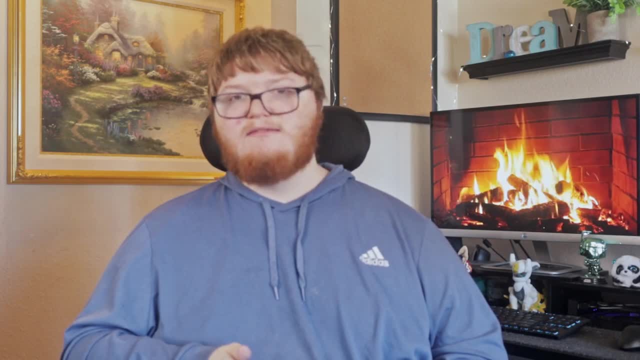 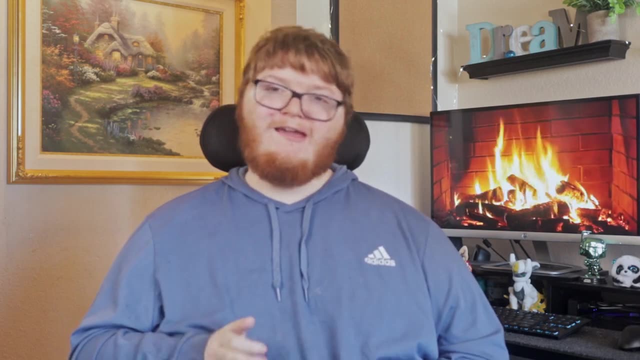 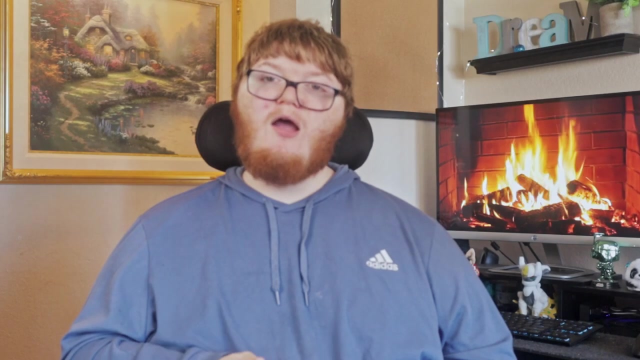 wanted to. If you missed the previous two videos in this series, the links to those videos will be in the description below. And, with that being said, let's get into it Again. we're back to asking the most basic question: What is world building? World building is the process of 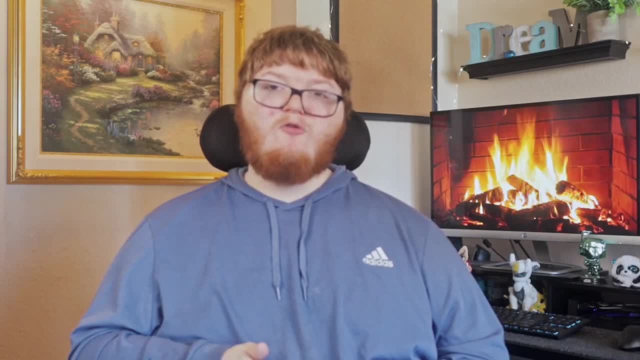 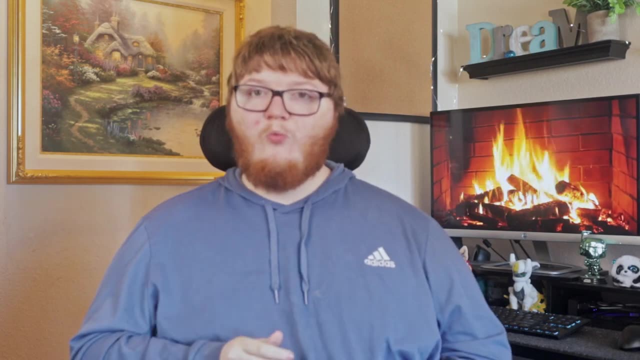 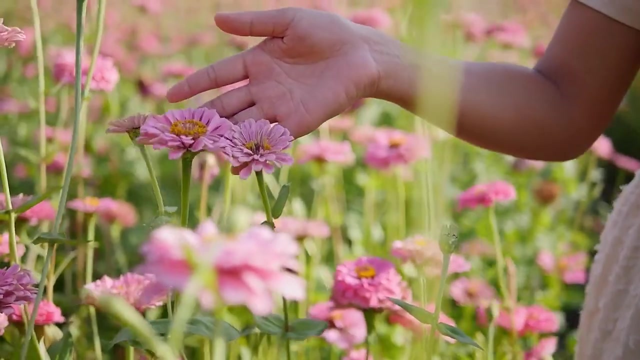 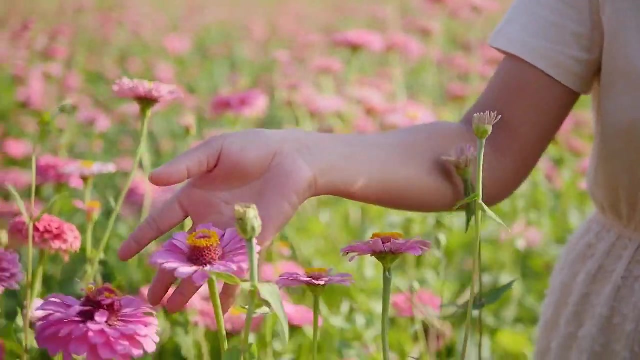 creating fictional settings or worlds, either within our own world or within an entirely new world created completely from scratch. World building in its most basic sense is just creating a setting. So your setting could be an entire new world that you create. It could be a house in some city, It could just be an. 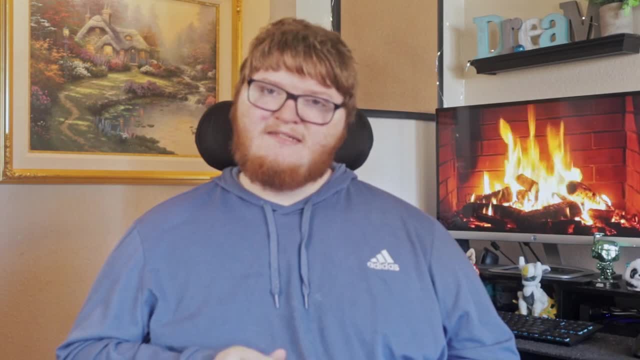 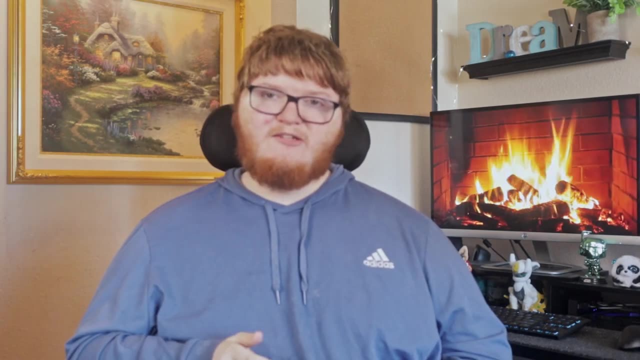 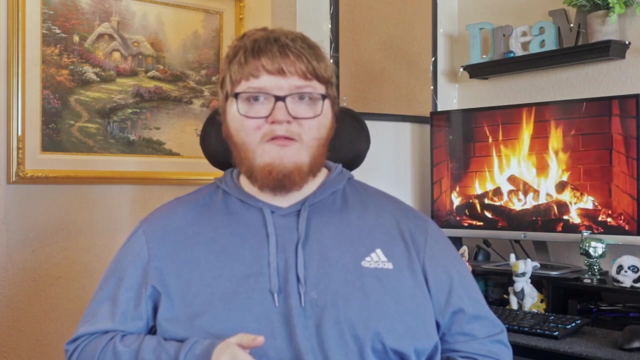 entire city on its own. If you build a city or a house that does not exist in reality, you are world building. So if anyone tells you creating something on the earth as we know it is not world building, they are completely wrong. As long as you build something new in the world. 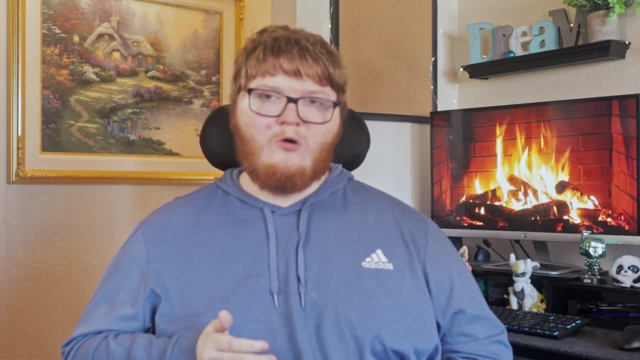 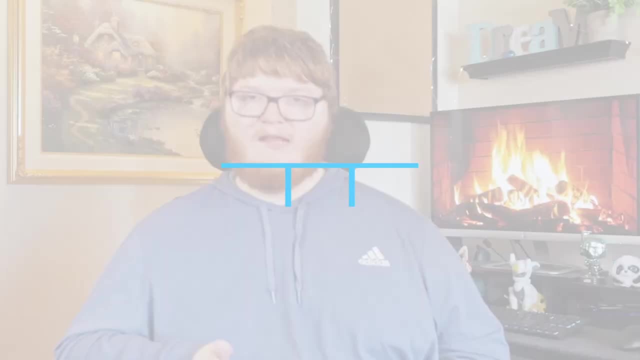 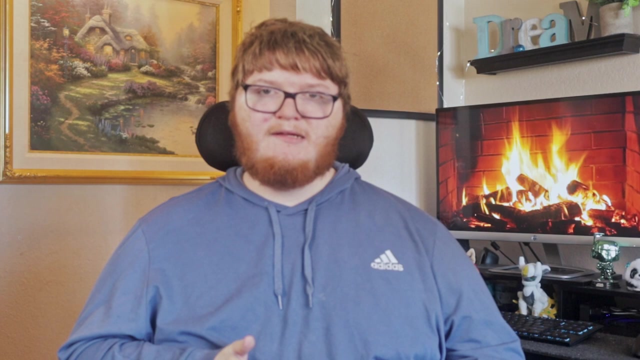 or add something to our world. you are world building. Speaking of that, we're going to move on to the types of world building. You have two different kinds of world building. You have primary world building and you have secondary world building. Primary world building: 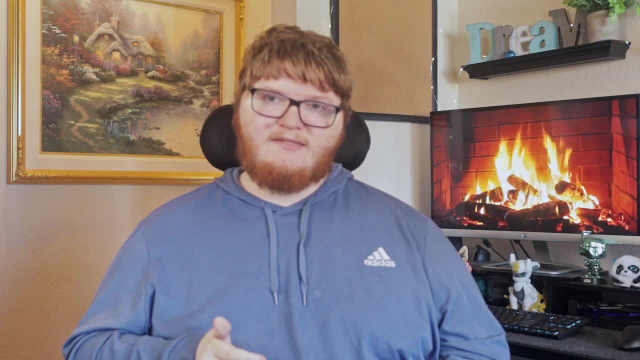 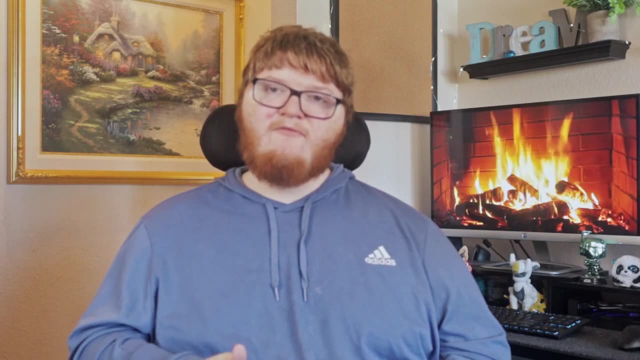 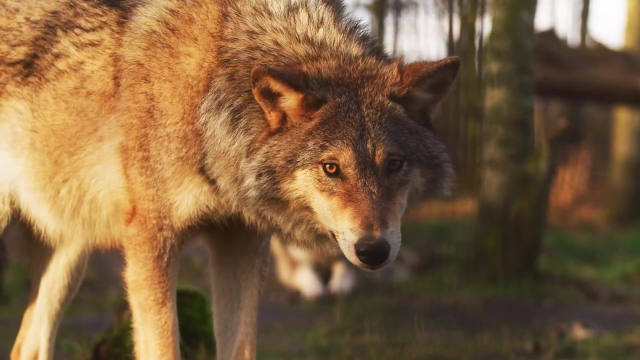 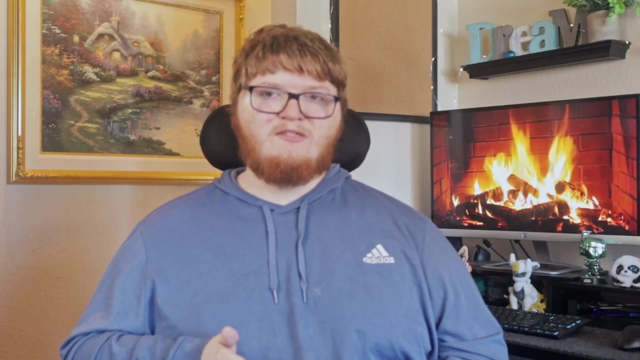 would be using our world and adding something to it. This fits into the low fantasy category, which also has contemporary fantasy, And then, even further down, you have urban fantasy like Twilight or Harry Potter. You also have alternate history books like Man and the High Castle. That also fits into. 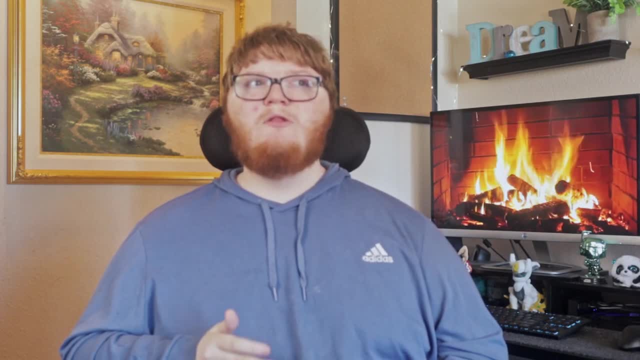 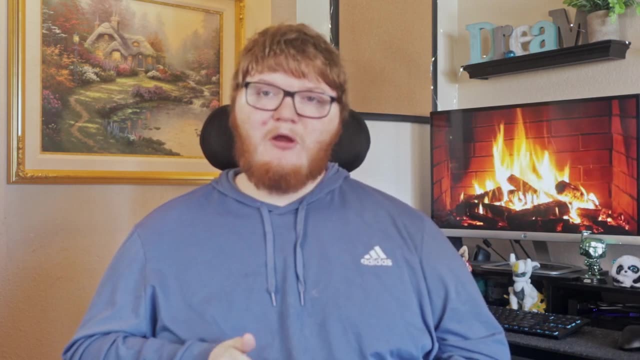 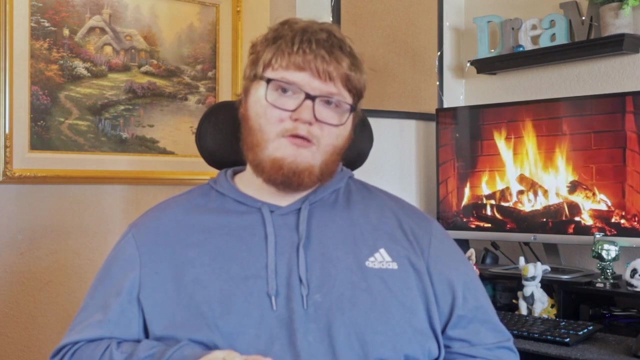 primary world building because you are building what could have happened. Now we get to learn about my favorite type of world building. Secondary world building is when you build the world from scratch and it's completely new. It's not Earth in the future or in the past. 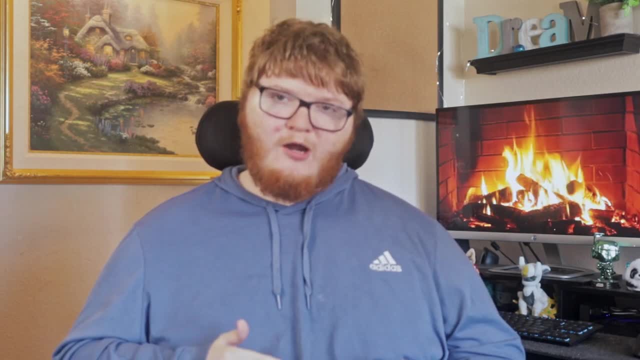 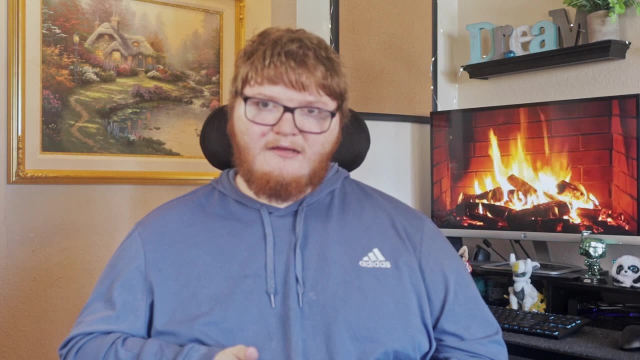 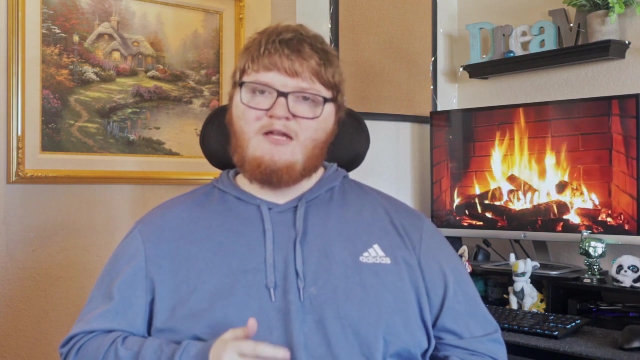 It's somewhere completely different from where we are now. This comes with high fantasy, and high fantasy is my favorite kind of fantasy because you get all this freedom when you're writing it. It's not you're stuck with the rules of this world. You can create completely new rules. 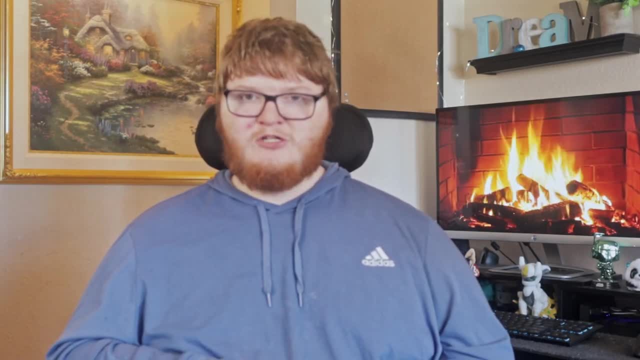 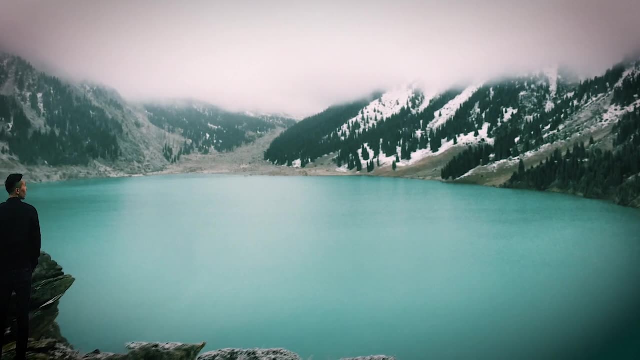 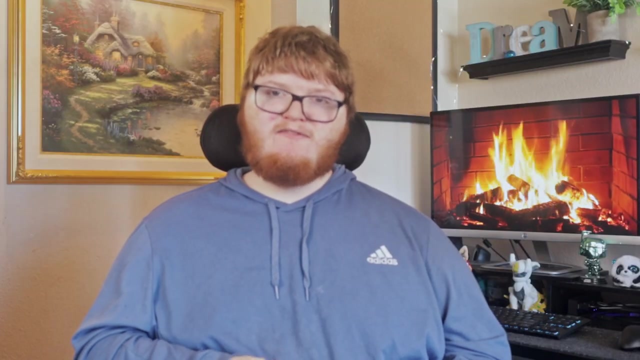 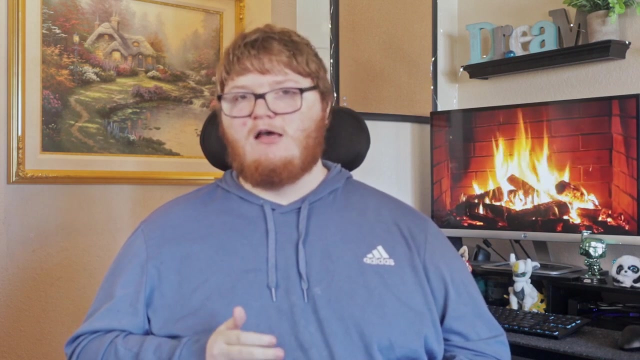 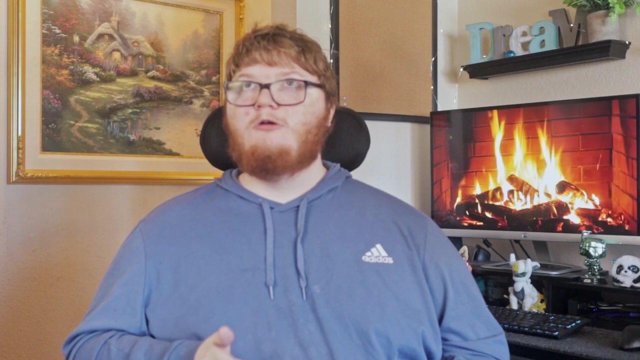 These completely new rules can change everything. You don't have to stick with the physics of Earth or anything that we know. You can completely change everything. Secondary world building just gives you so much more freedom and it's really fun to create these things that come together to make either high fantasy stories like Game of Thrones or other. 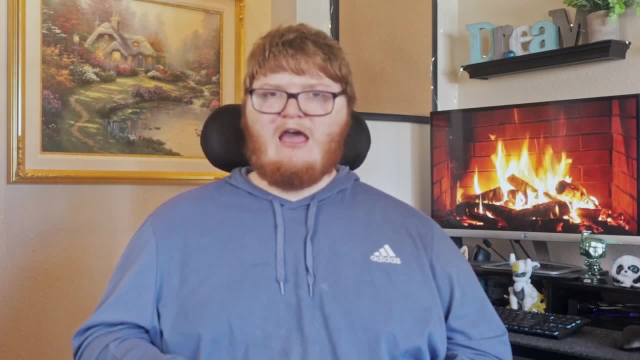 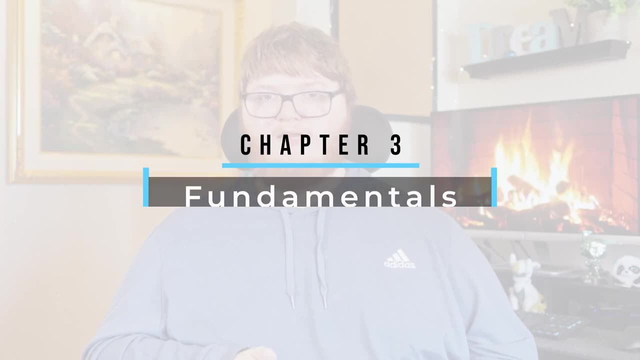 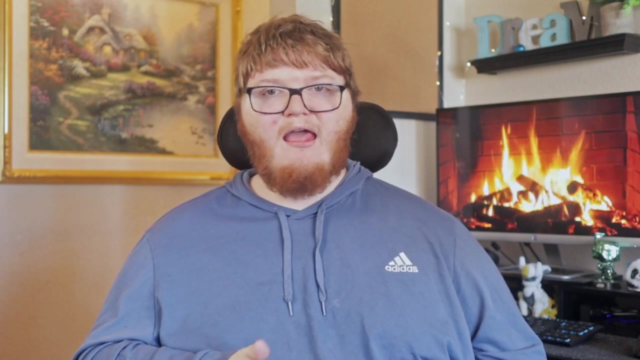 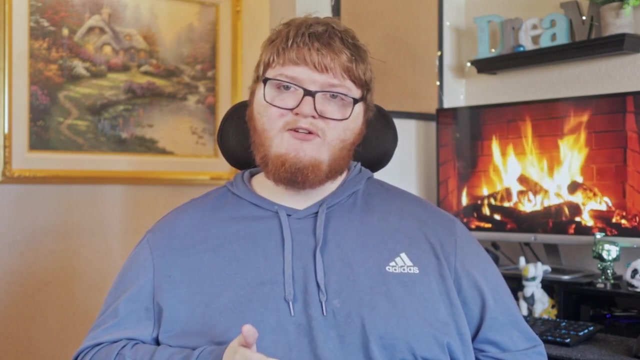 stories like space operas with Star Wars, where you have thousands of different planets to explore. Now we're going to move on to the fundamentals of world building, and there are five fundamentals of world building. These fundamentals can be mixed and mashed together to create a different structure for you, but this is how I personally work through world building. 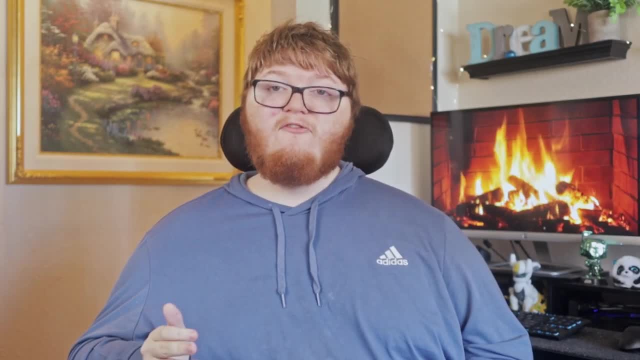 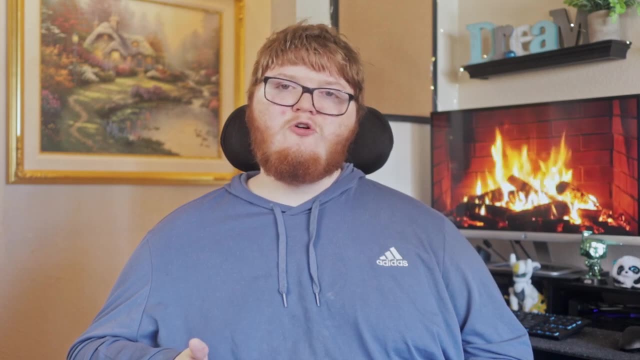 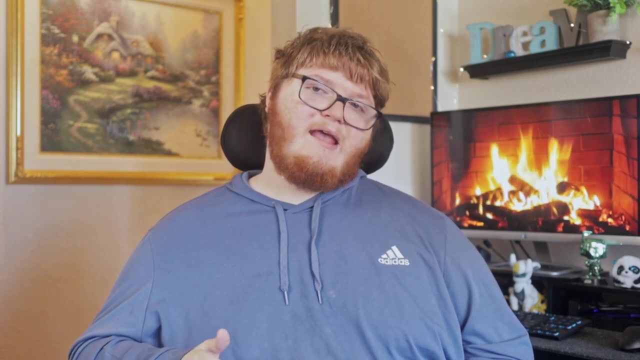 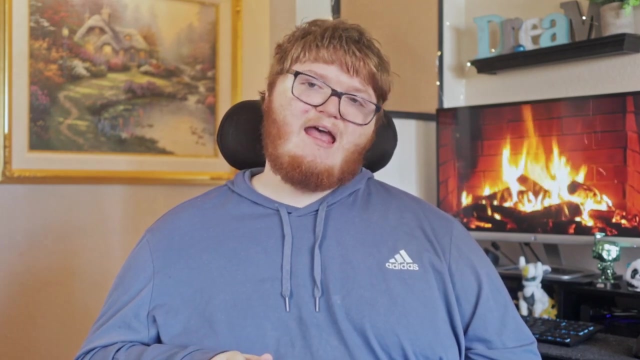 and I always start with these five things. The first, fundamental, is geography. Geography encompasses everything about the physical world, Your landscape, your climate, your flora and your fauna. These things and more come together to build the geography of your world. They need to exist outside of this world if you do indeed create that new world, Of course. 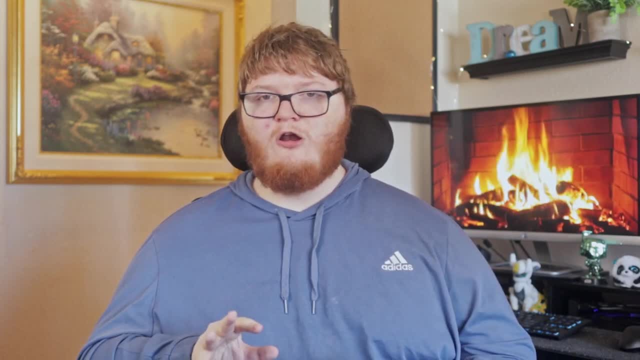 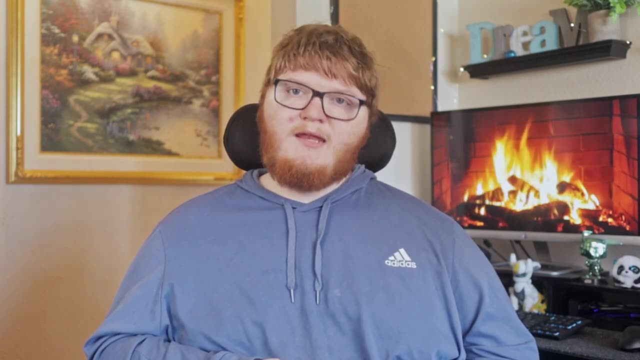 your geography can be completely different than what we have here on Earth. The second fundamental of world building is people and politics. People and politics include government, languages, races, economy, stuff like that. People and politics are the same thing. People and politics are the same thing. 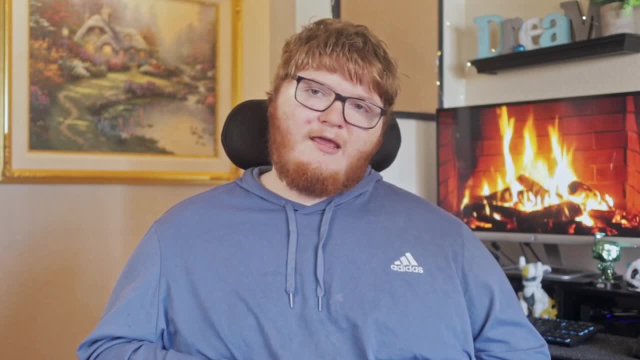 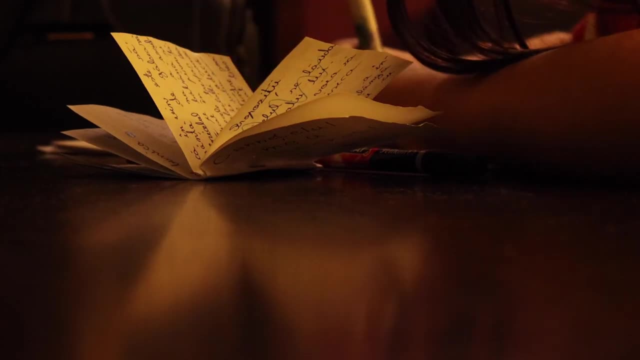 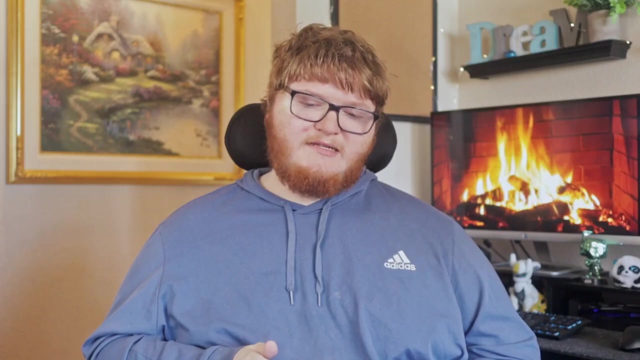 Obviously, if you're not writing a political thriller, you don't want to put all your time into politics and people. If you're not really going into it, there's really no point- And that can be said for all of them- If you're not going to use one of these fundamentals. 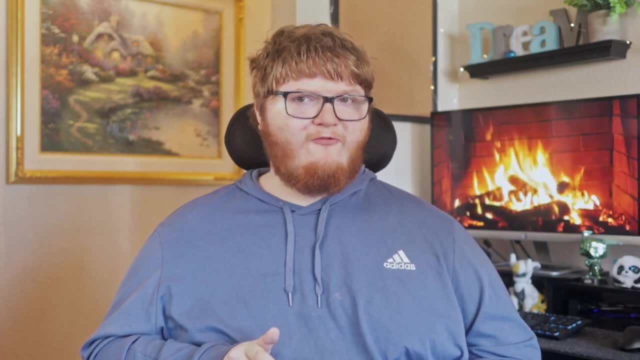 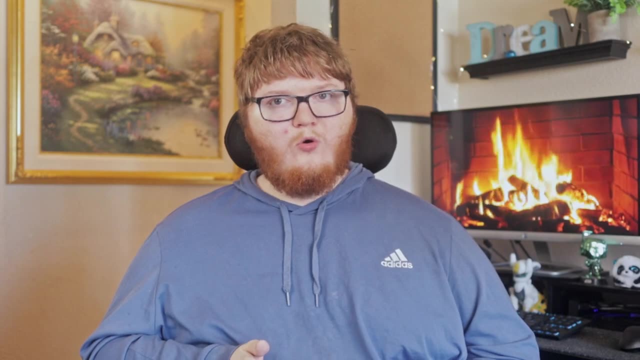 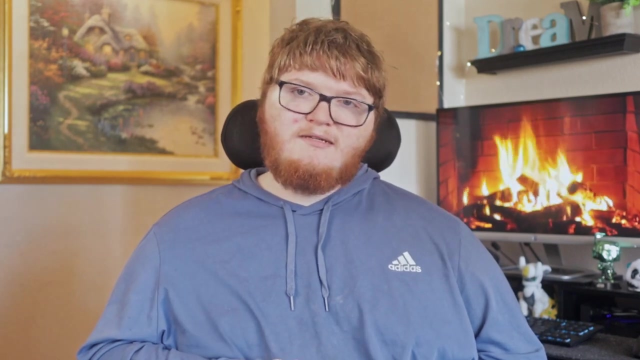 a lot in your story and don't focus on it that much, then you don't HAVE to put it in your story or even build it up that much. The third fundamental is culture. Your culture includes art, like paintings and drawings, and architecture. 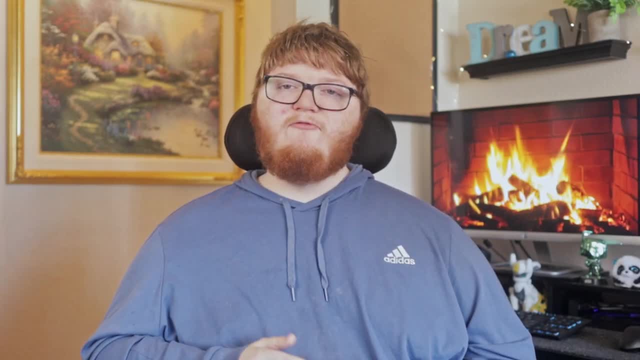 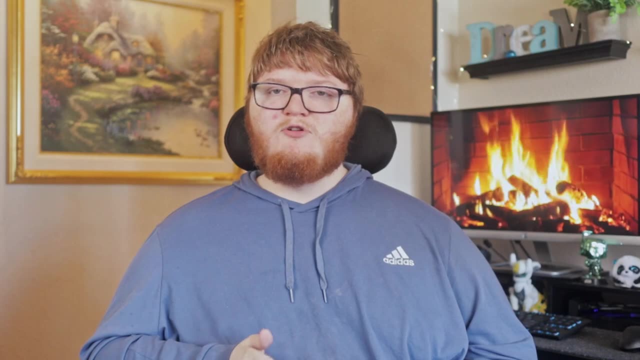 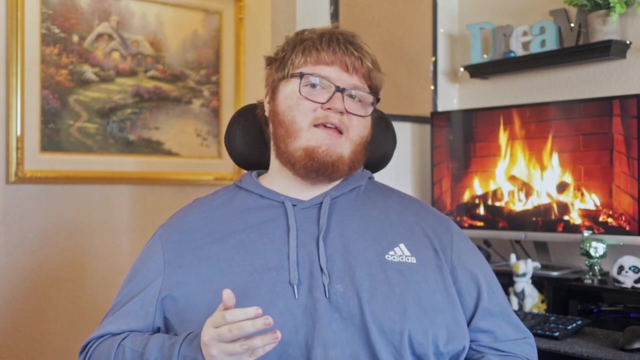 It also includes your social rules and your religions. I have known people to come up with a completely new pantheon of gods. I've seen people come up with multiple different religions in one story because they just have fun with creating things like this. The fourth fundamental is history. 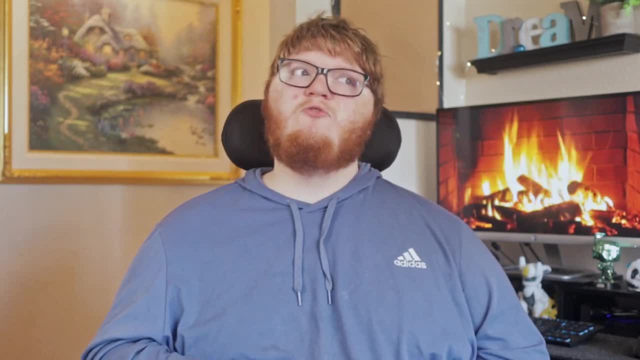 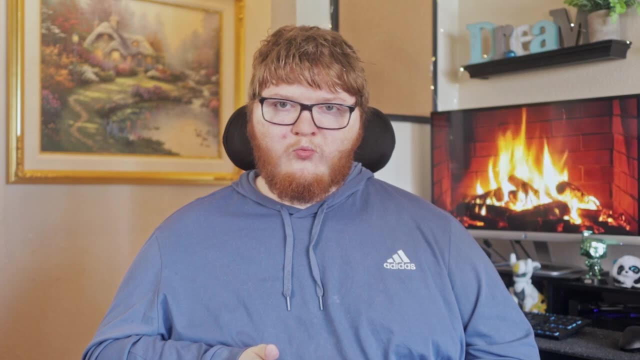 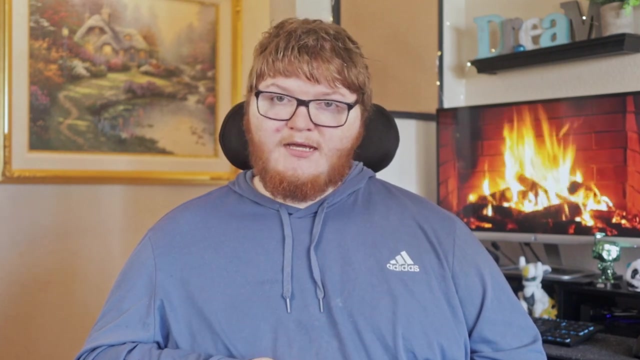 History includes the world history. what has happened throughout history from before documents are being made about the history of the world. Could some of your world history be shrouded in mystery that no one actually completely understands? Your history can also include power shifts. 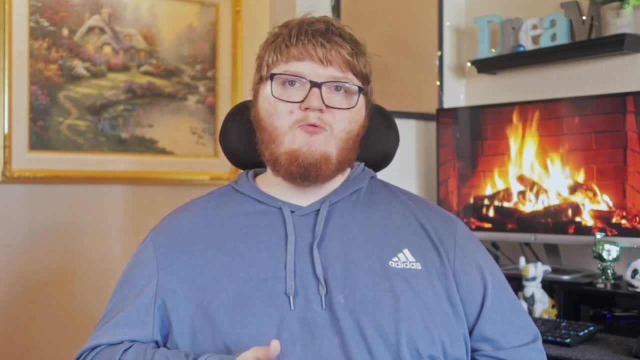 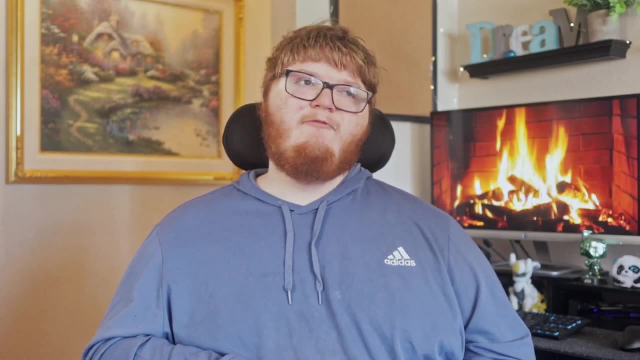 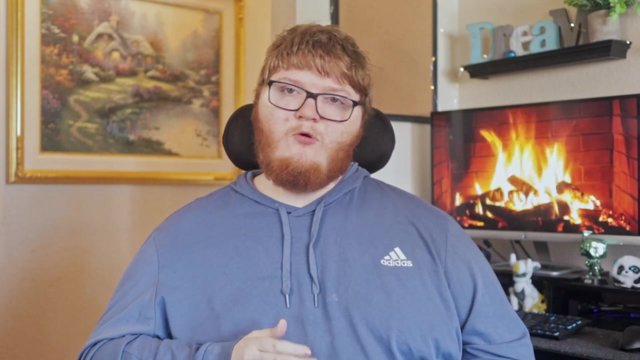 like: what races have power at what time? if there's been any coups in your history, if there's been one kingdom that has risen and fallen to power, Then you can also go into recent and ancient history. what has happened recently to shape the world? 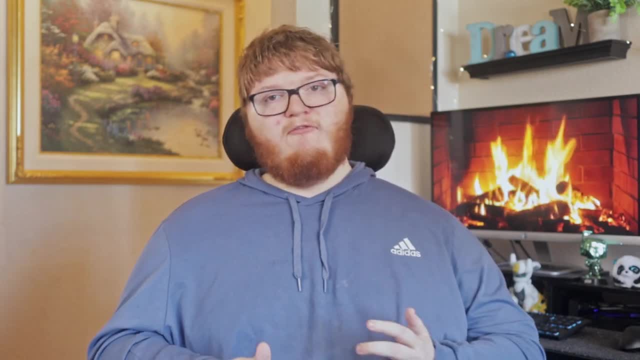 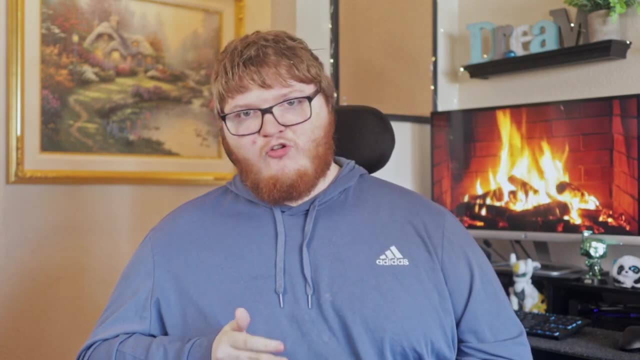 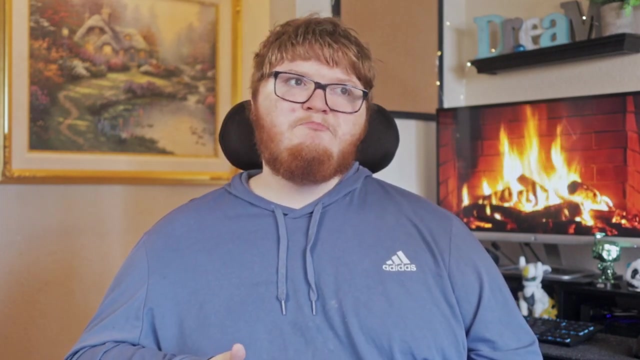 what happened in the ancient world of your world that caused things to happen as they are happening in your story, As you write it. The fifth and final fundamental of world building is magic and technology. This is the most self-explanatory part of it. 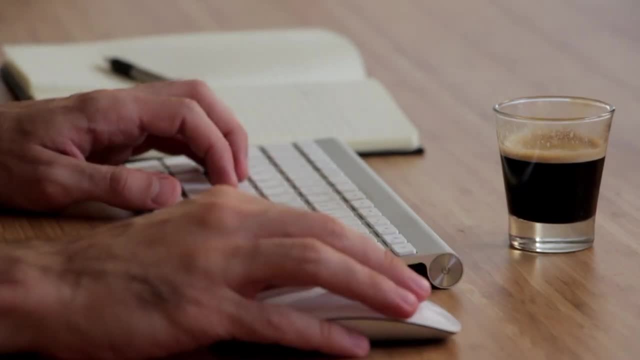 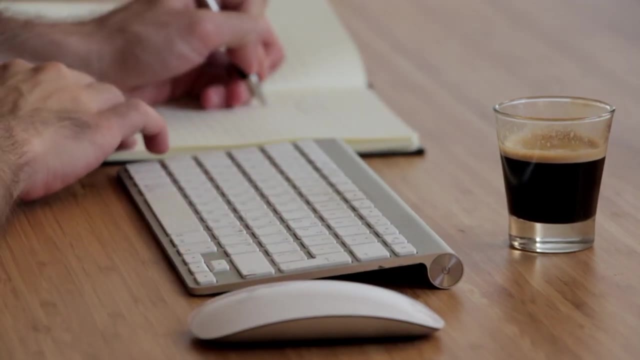 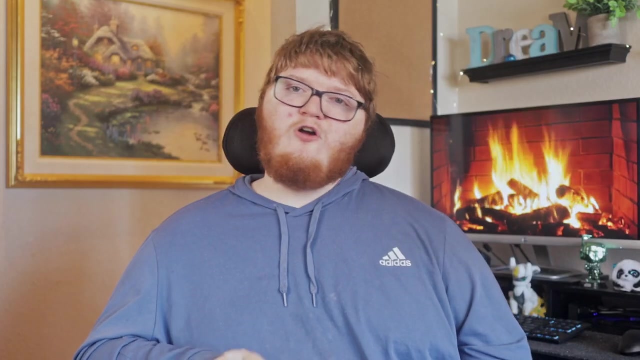 If it's applicable to you, you need magic, But if it's not applicable to you, you can just skip over magic completely. And then it also covers technology, weaponry. it can cover medicine, it can cover all sorts of things. You could have guns, you could have swords. 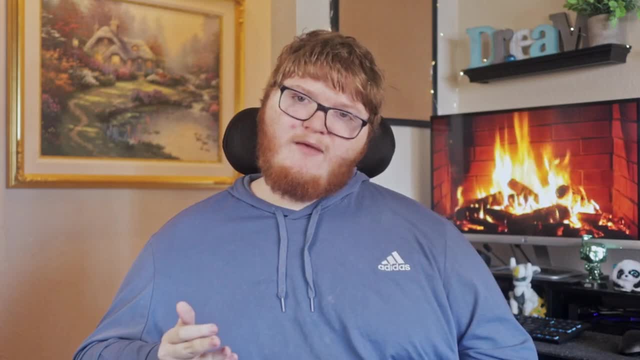 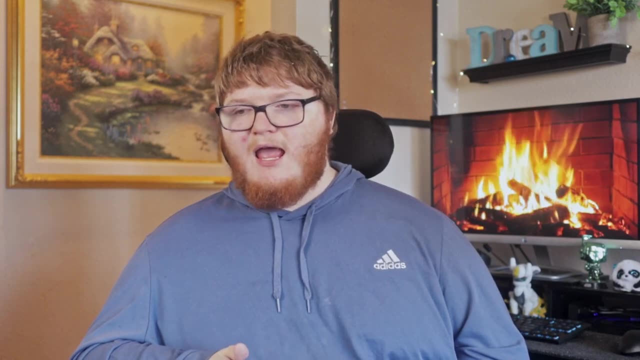 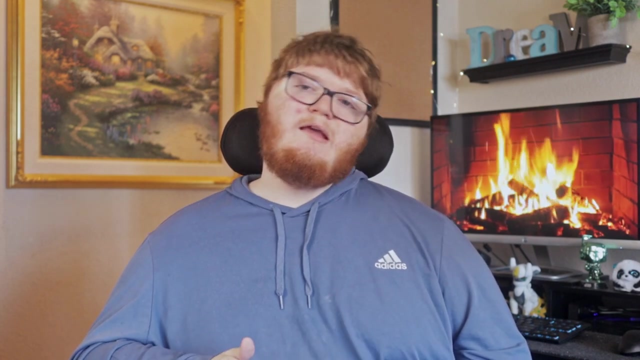 you could have herbs, you could have modern medicine, future medicine. It's all over the place. You can make this stuff up as you go And that's part of the fun: Just coming up with these things to put into your world. 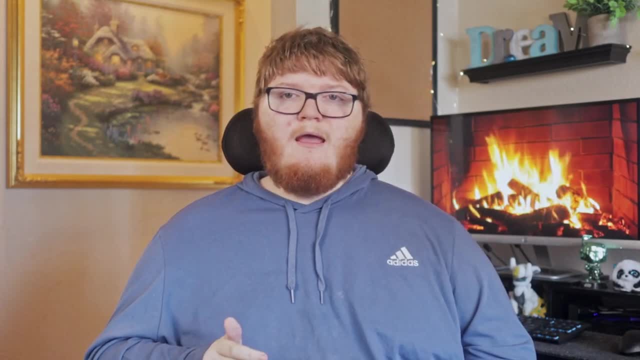 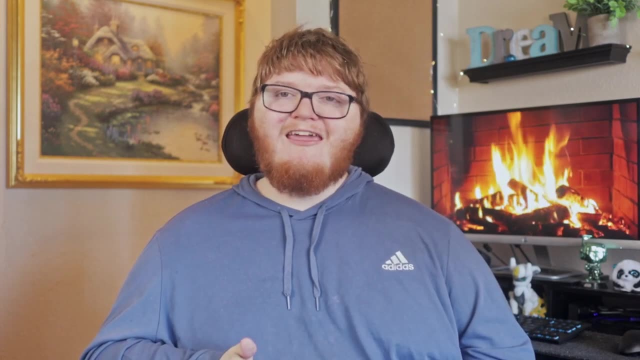 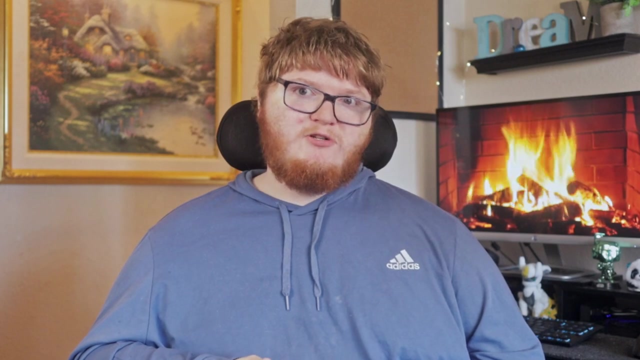 And not all of this will make it into your story And it could just be happening in the background And that's perfectly okay. There's nothing telling you that you have to have all of this in your story. Like I said earlier, you could skip any of this. 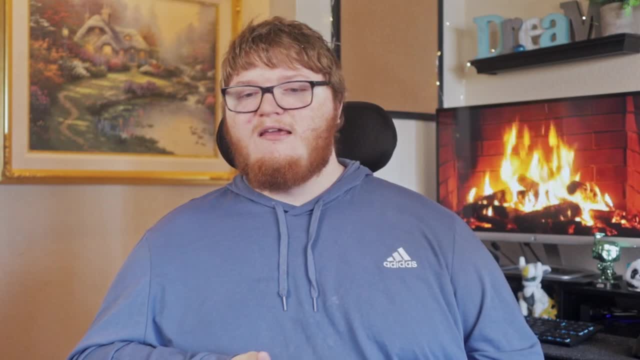 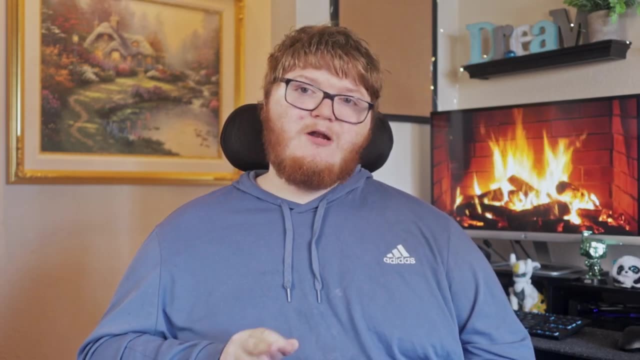 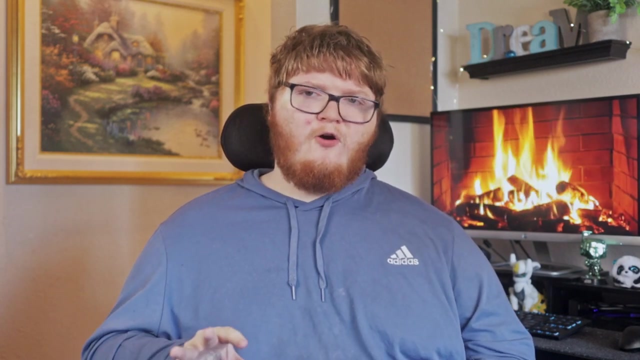 or you could do all of it, But really my suggestion would be to take one or two of them and roll with those, And what I mean by that is choose magic and weaponry and geography and use those as what you build, Build most. 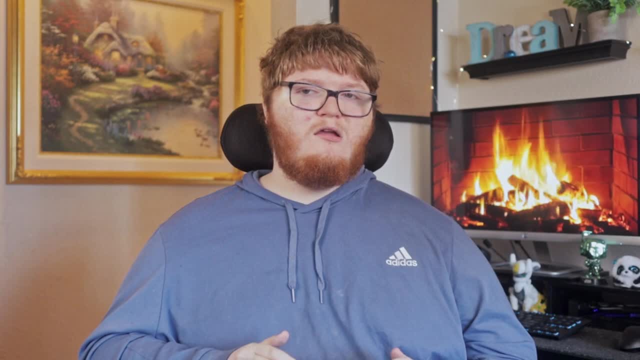 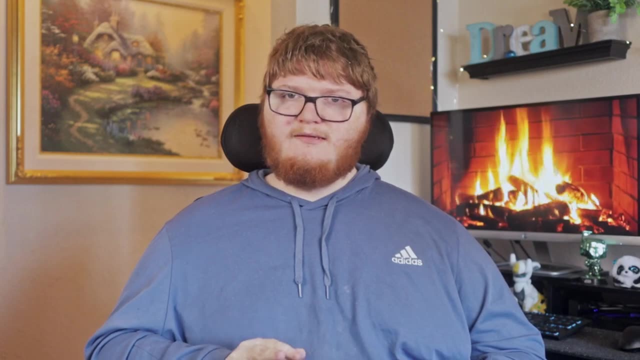 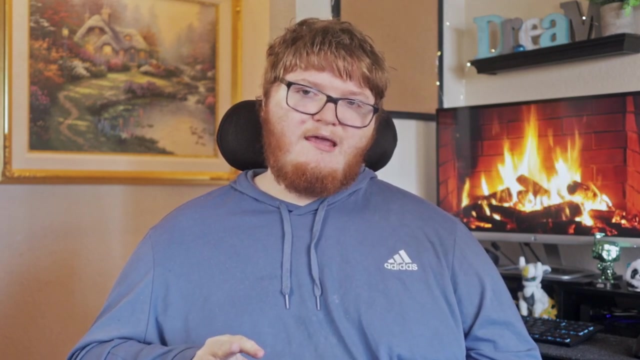 You don't want to be caught in the world building hole too long, Which is why I don't suggest you do all of them in every single world you build. You can do all of them, but take one or two and use those mainly as your big stepping stones. 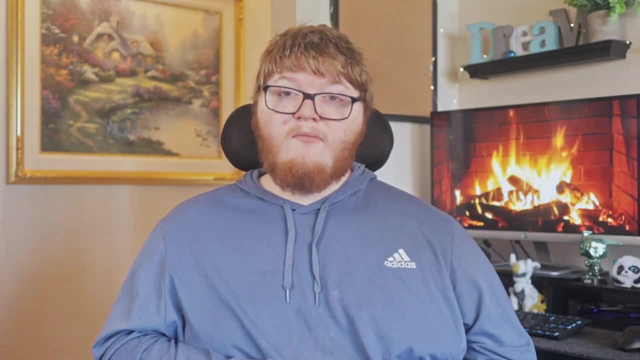 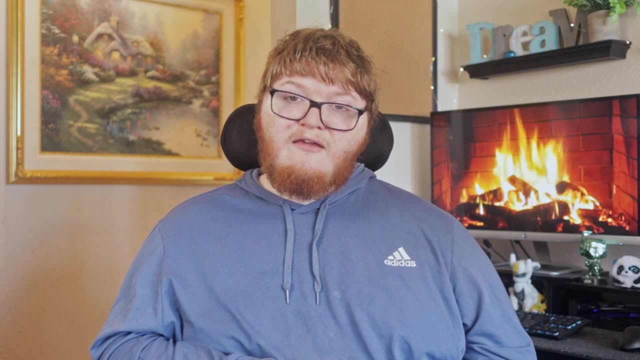 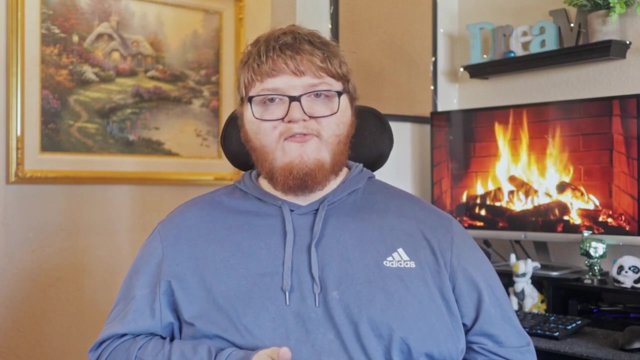 for your world building. Finally, we're gonna talk about why world building is important to your narrative. First reason is that effective world building enhances the narrative, including the plot and the characters, And that's why it along with plot and characters. 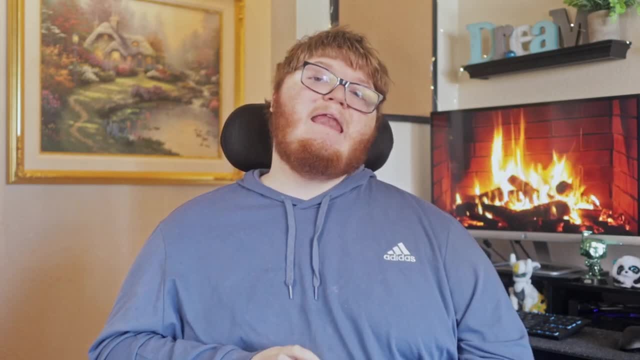 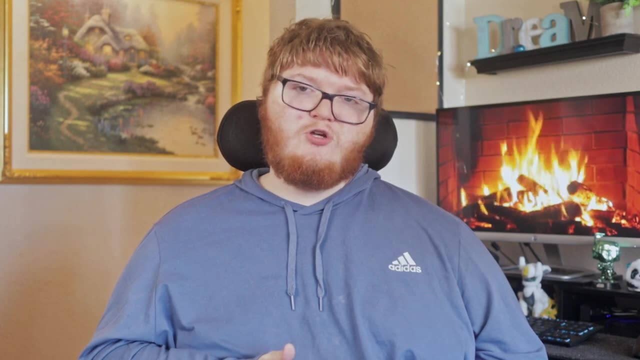 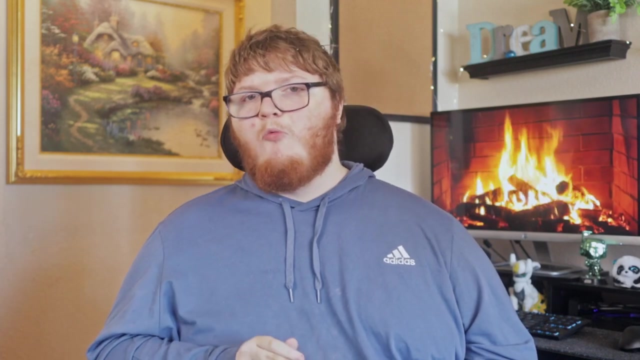 are the three fundamentals, Because they work hand-in-hand. Without the effective world building, your world will be dull and it won't capture your readers as much as you might want it to. This leads directly into my second point, That is, that world building. 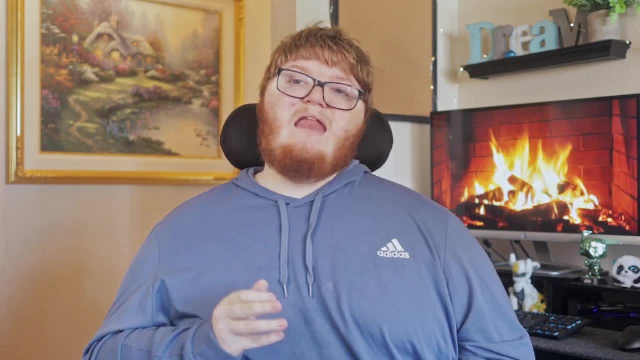 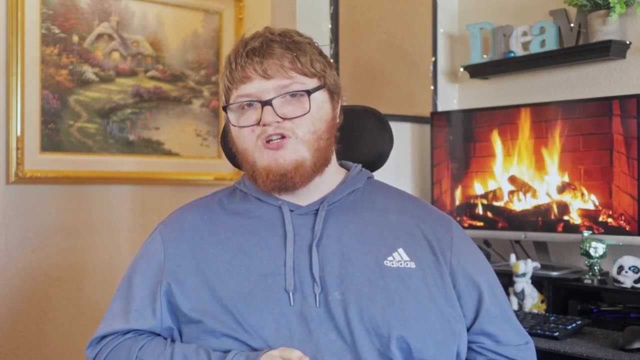 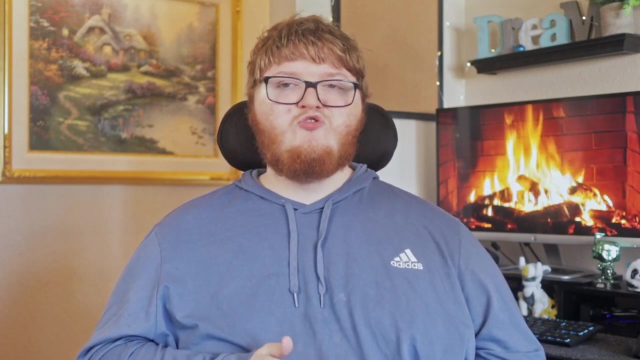 can trap your readers in the world and make them feel like they are actually in it, experiencing these events. This is one of your most difficult jobs as a writer, And that's because it's really hard to capture readers' attention nowadays. People have shorter attention spans than they used to. 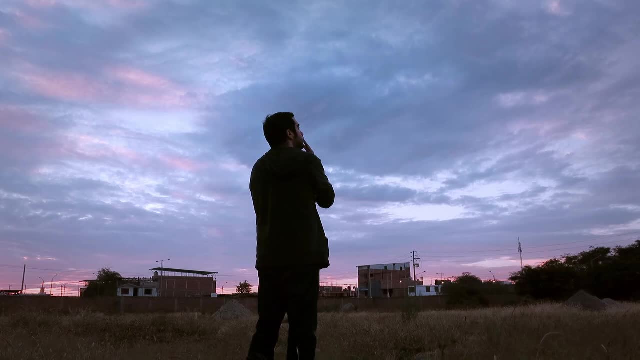 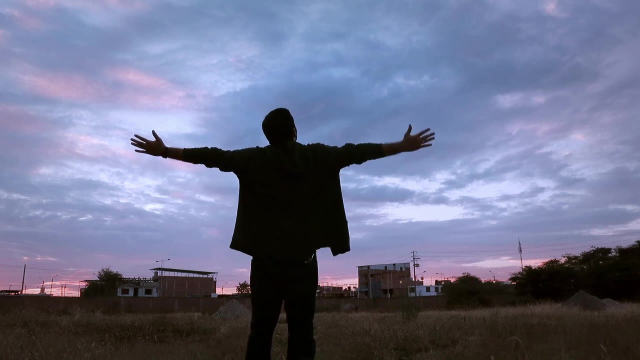 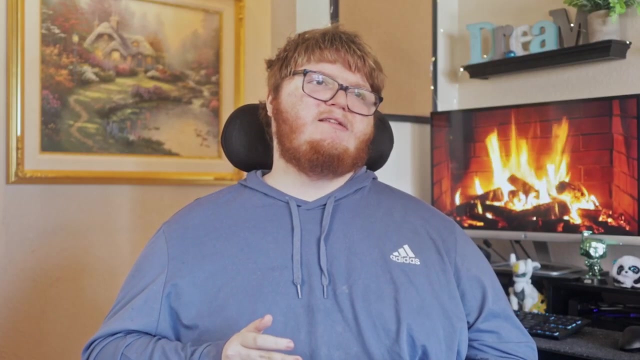 But once you get them engrossed in your world, it's difficult for them to escape it when they're reading your story. My third reason for why world building is important is that world building gives your narrative somewhere to take place If your world building doesn't have a place to.